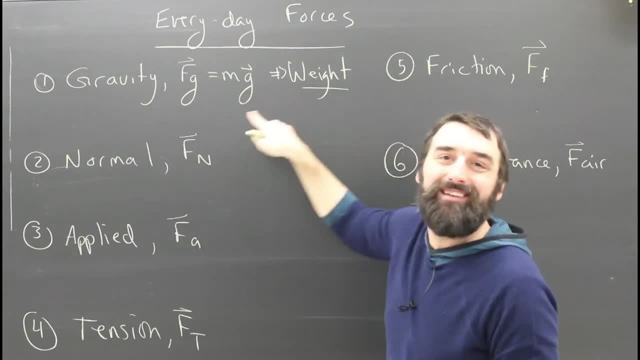 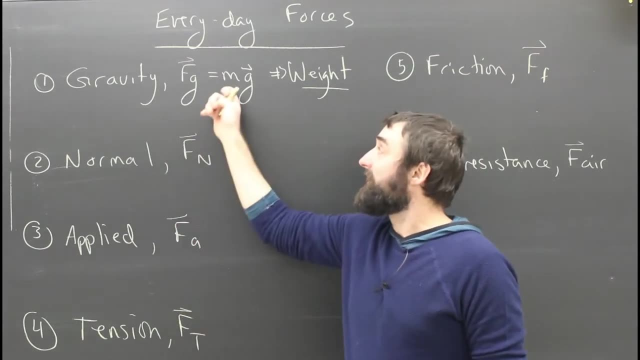 force of gravity m times 9.8 is the weight. Weight and mass are not the same thing in physics, even though in everyday life we might say I weigh 90 kilograms. It doesn't make any sense: Kilograms, 90 kilograms. 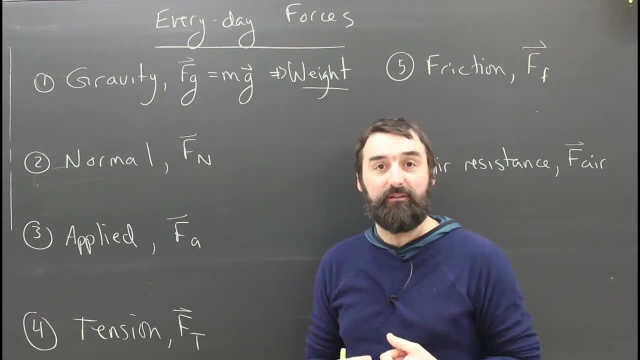 is how much inertia I have, how much resistance I have to acceleration, how hard it is to push me around. It's also proportional to how hard the Earth pulls down on me. That's my weight- a little less than 900 Newtons. Weight is a force. It's measured in Newtons. 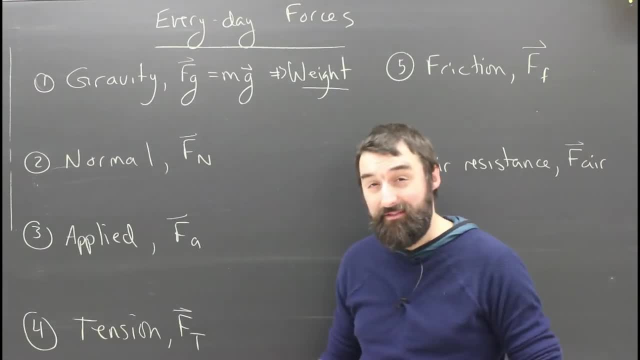 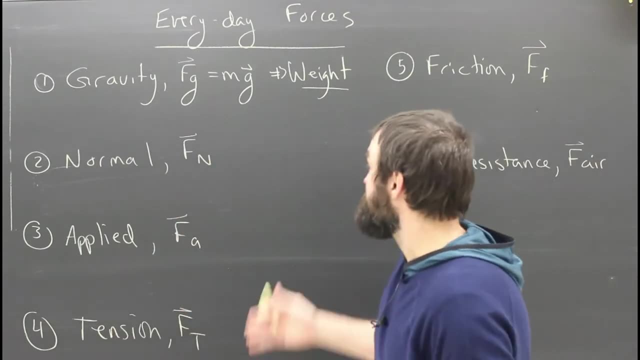 Mass is a resistance to acceleration. It's measured in kilograms. They're not the same thing. What are some other everyday forces? So the normal force, You guys are familiar with Fn, If something is on a surface, like, let's say, we have a table and there's a block sitting. 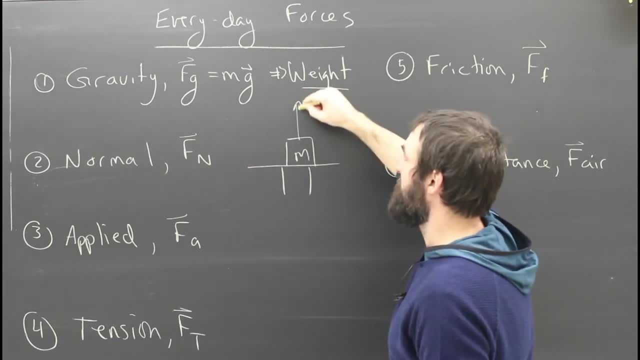 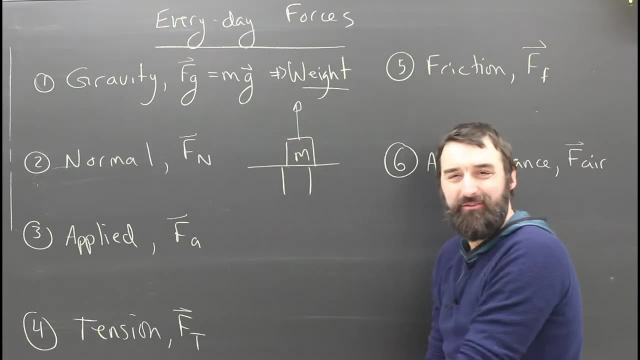 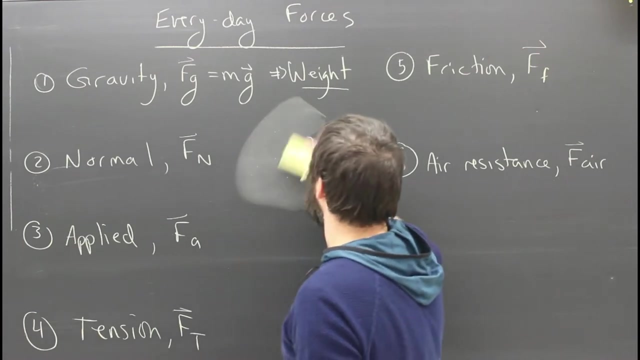 on the table. the table is pushing up on the block. It stops it from falling through the floor. If the table didn't push up on it, gravity of course would pull it down and it would sink into the table. But it doesn't, and that's because of Fn. So the normal force. 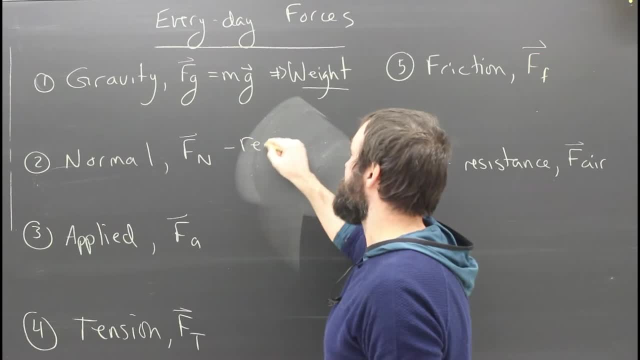 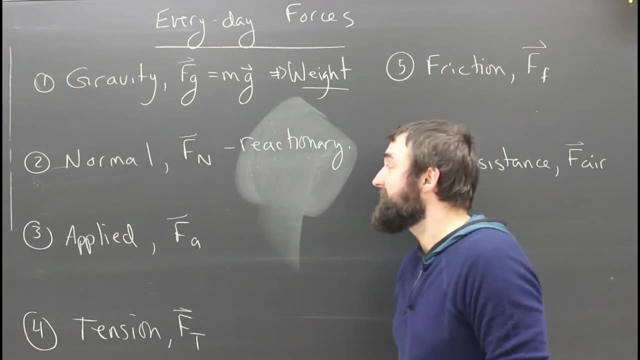 Fn has no formula, but it's kind of reactionary. It's as big as it needs to be. It's reactionary- I'm not sure that's how you spell- reactionary. It's as big as it needs to be. It's called. 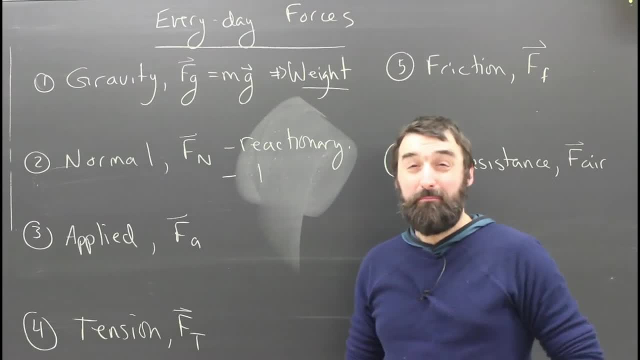 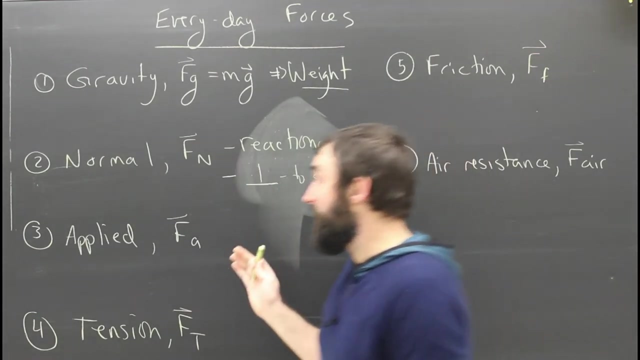 the normal force. Normal is a fancy math word for perpendicular. It's called the normal force because it's always perpendicular to the surface. That's why it's called Fn. There's a lot of interesting things about Fn. Sometimes it's equal to gravity, but it is not always. 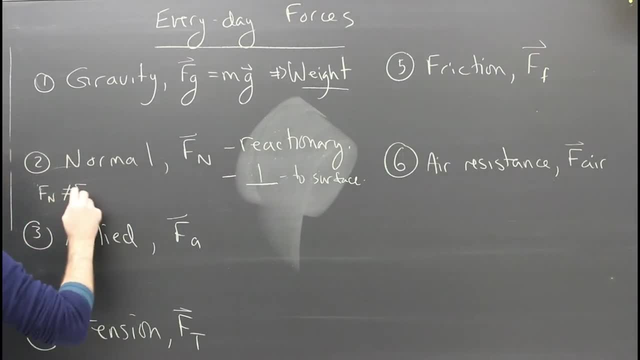 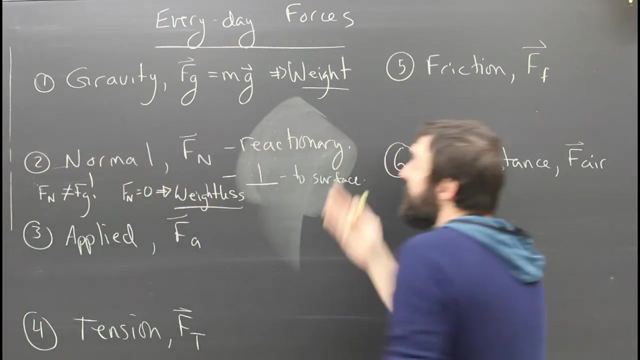 In fact I'm going to write: Fn is not equal to gravity. I should say not always, because it sometimes is, but it is not always. Another interesting thing about Fn: if Fn is zero, if we have no Fn, then we are said to be weightless. And that's interesting to me because the weight 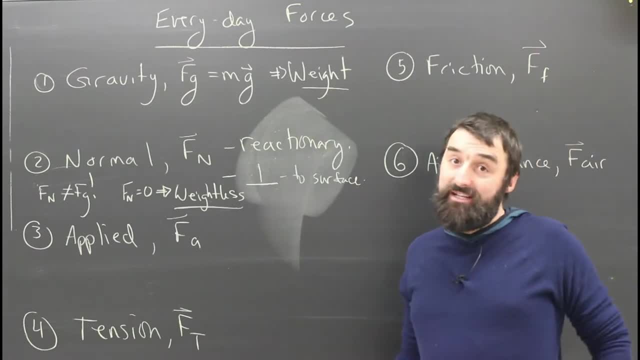 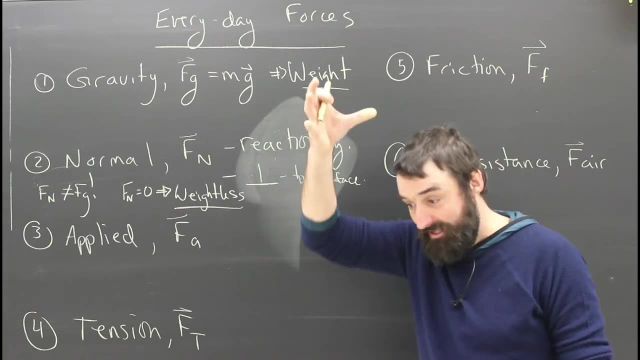 is Fg, so you could be forgiven for thinking that if you are weightless you have no gravity. that's not true. If I put Mr Carawan in an elevator and I cut the cable, he falls In the elevator. he is falling at 9.8.. Gravity is causing him to fall, but there's no normal. 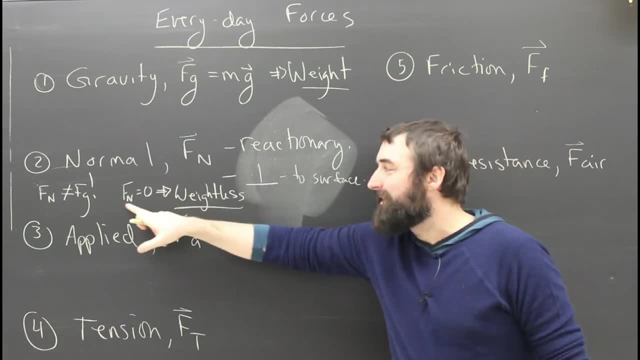 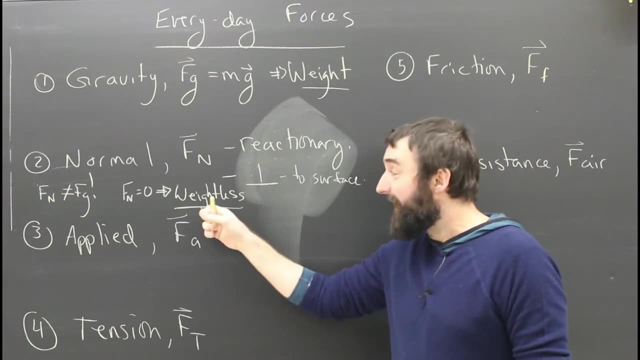 force He feels weightless. Fn is kind of how heavy we feel. We'll talk more about that later. If Fn is zero, it's weightless. Fn is what a scale measures when it tells us our weight, our mass. Well, okay, So we'll learn more about that later. 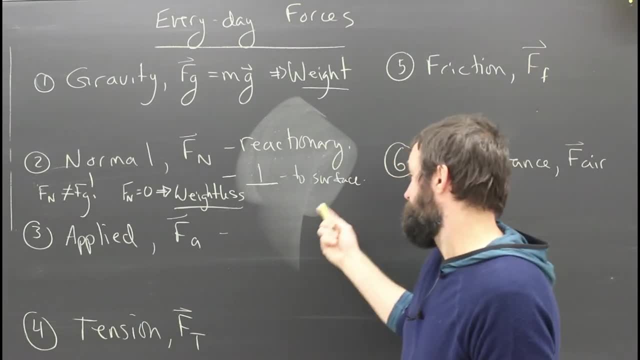 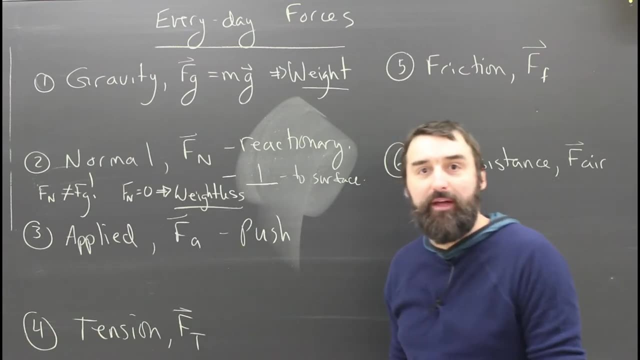 Side force: Fa any old boring push. If the question says the dude is pushing a box across the floor, the dude is pushing, let's call that Fa any old push. Simple, not much to say about that. What about tension Ft. if there's a rope? if I put a rope around something? 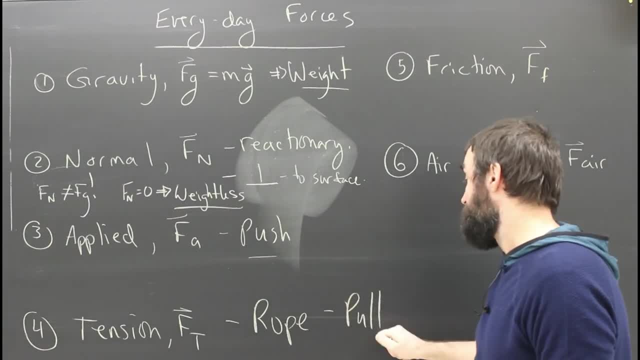 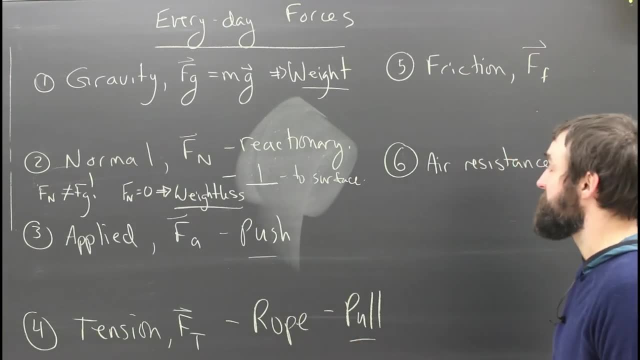 and I pull it, then we'll call that tension. Ropes can, of course, only pull No big deal there. It's pretty easy. There's no formula for it exactly. In the different situations you'll just have to figure out how big it is. It's pretty straightforward. 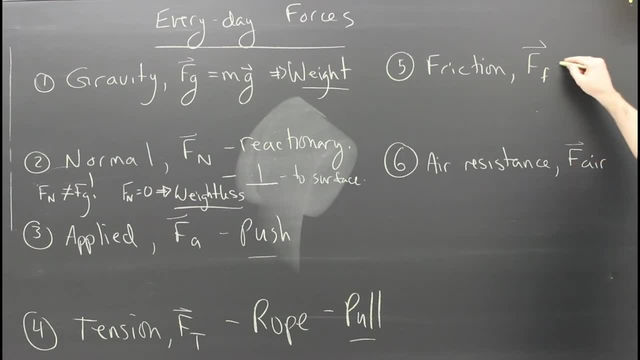 A more interesting one: friction- Friction. we'll talk lots about. Friction has a very important goal: It tries to fight, not things moving, but it tries to stop things from slipping or sliding or skidding. So it fights what I'm going to call slippage: It tries to stop. 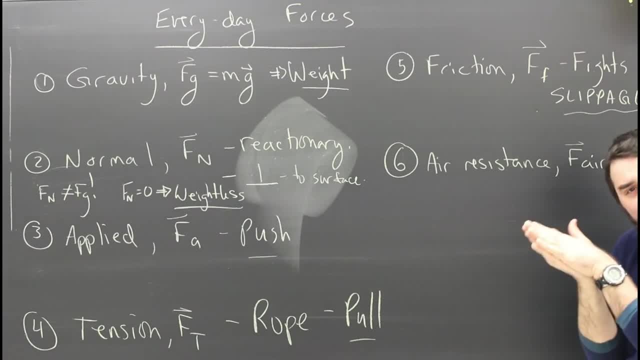 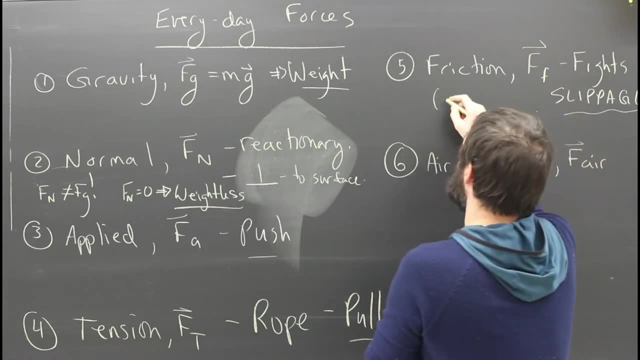 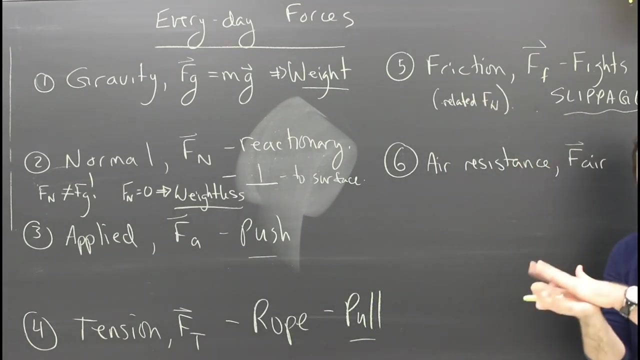 relative motion between two surfaces. Slide Rope have to be in contact And in contact means there's an FN. So friction- we're going to learn later- is related to FN. That's important. When things are touching, there's friction. If they're not, 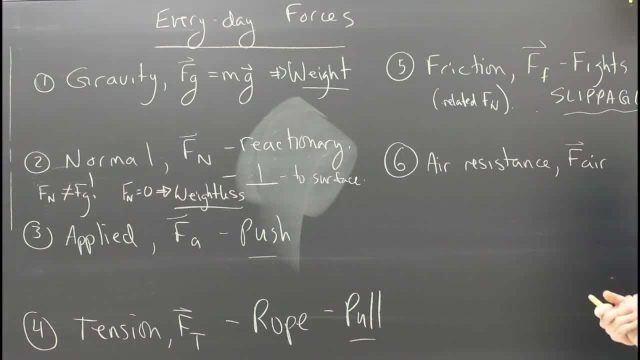 touching, there can't really be friction. It fights slippage. We're going to talk about that. There are two types. We'll talk about that later too. There are two types. Another common force is air resistance. The formula is not something. 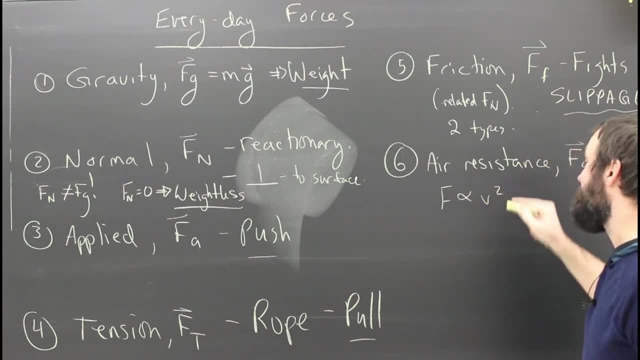 you need to know at this stage, but it is interesting to realize that it's related to speed squared. So the air resistance does oppose motion. Friction doesn't oppose motion, It fights slippage. But air resistance opposes motion. It opposes.